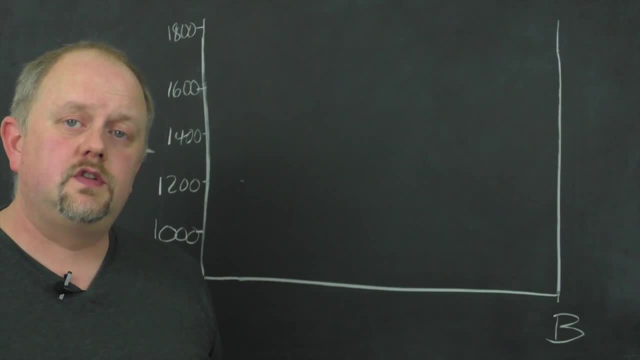 AB4, which is stable between 1000 and 1200 degrees C. and then we're given two eutectic points as well: E1, at 1300 degrees C, 40 percent B, and E2, 1350 degrees C, 80 mole percent B. 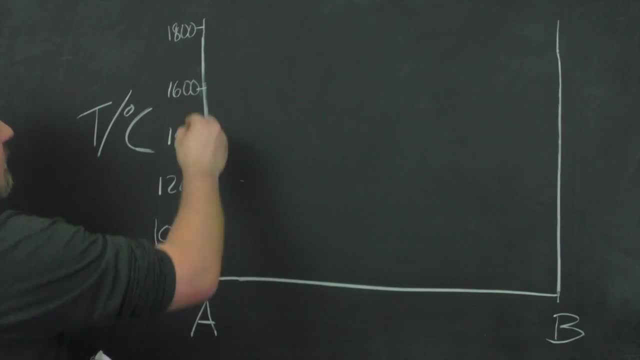 So let's have a go at writing that up. So we've got A, which we know melts here about 1750.. B, our component over here, melts around about 1650.. OK, Now, the one neat thing we have here is a congruently melting phase. 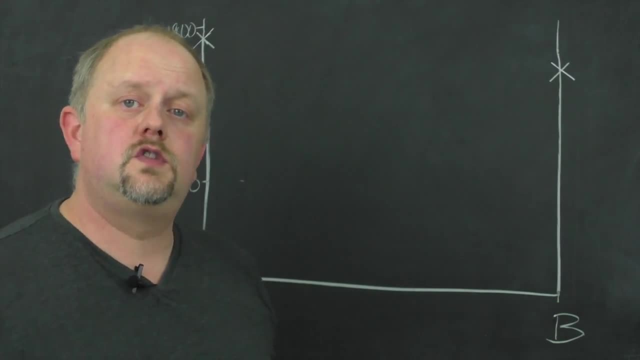 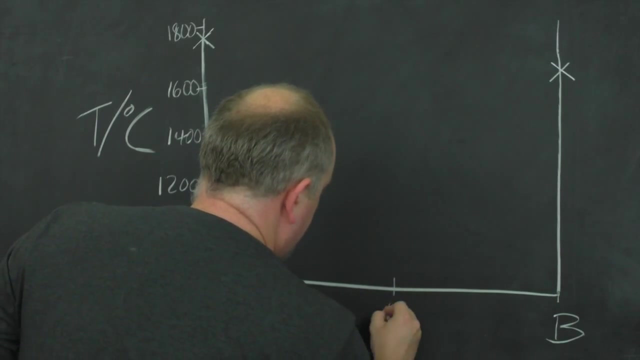 so let's deal with that first. Congruently melting phases can be used to divide the phase diagram into different sections. So if we have a phase in the middle here, which is AB, we know that mounts congruently at 1500 degrees C, which is. 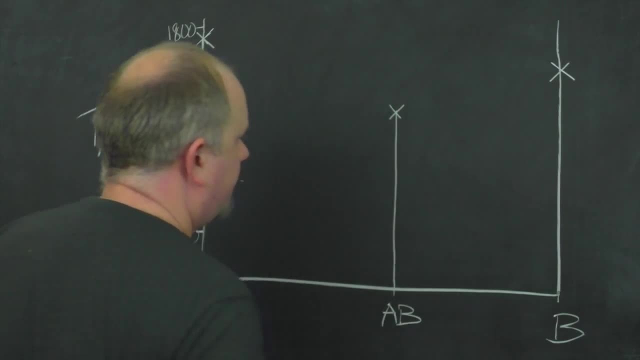 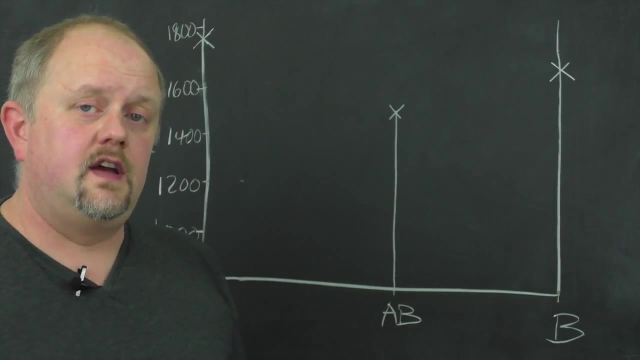 going to be about there so we can draw on that line. so, straight away, we've divided the system up into two different sections. we then know that we've got another phase, A3B, which mounts incongruently at 1400. so A3B is 25% B. 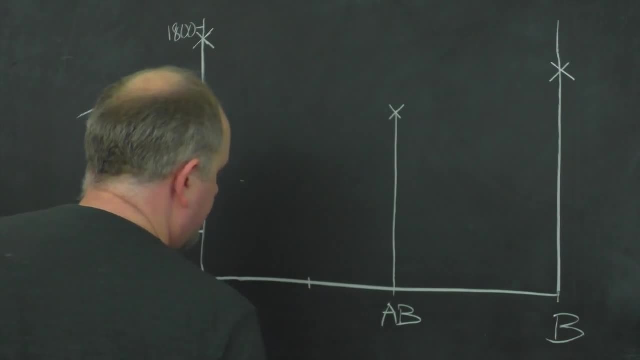 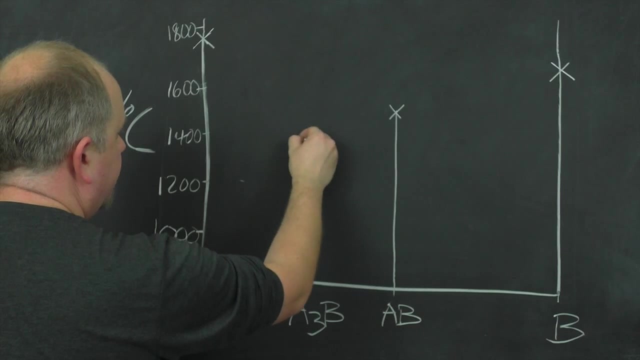 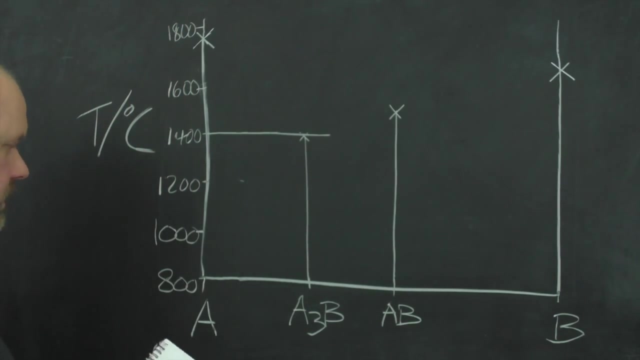 75% A, so it should be about here. so a 3B and that melts incongruently at 1400. so we know it's going to look something like that. ok, so we've got this classic T shape from an incongruently melting phase. Next we've got one final. 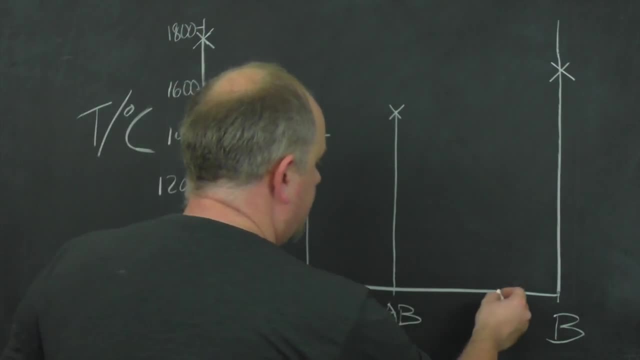 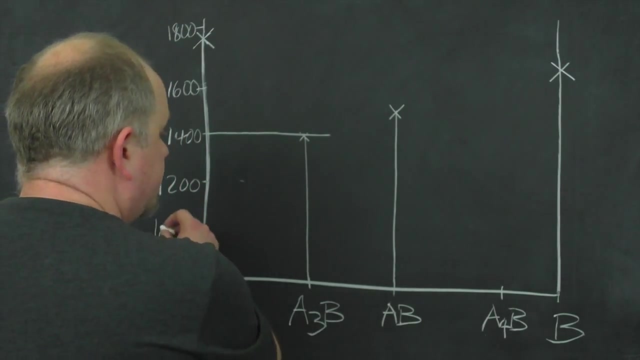 intermediate phase, which is AB4, which is 80% B, So we can put that somewhere over here. So A for B And we're told that that is only stable between 1,000 and 1,200 degrees C. This often catches a lot of people out when 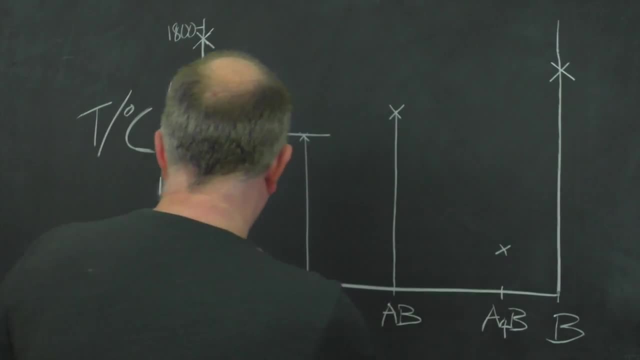 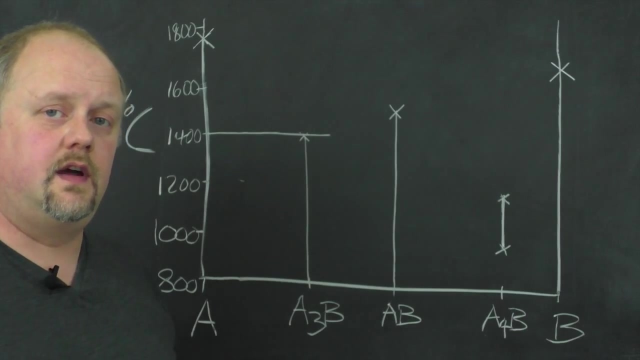 I do this sort of question. So 1,000 is there, 12,000 is there? So the line stability for this line phase only extends over that region, And that means that we can also draw on lines top and bottom. Okay, so we've then got two eutectic points. The first one is at 40 B. 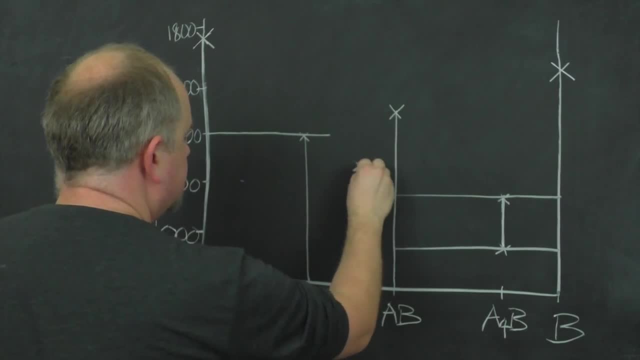 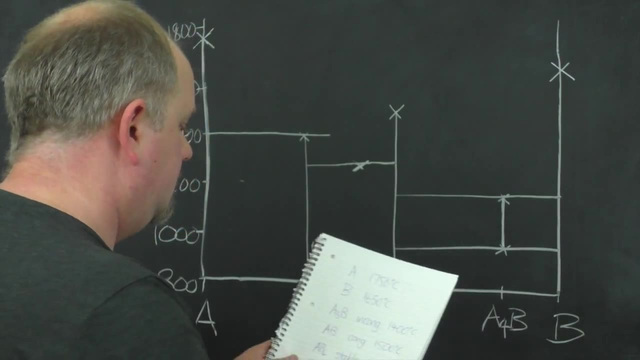 so somewhere about here, at 1,300 degrees, It should be about there. So if it's a eutectic, we've got a line going through it And another eutectic at 80 mole percent B, 1,350 degrees C. So that's directly above A for B. somewhere about there And again. 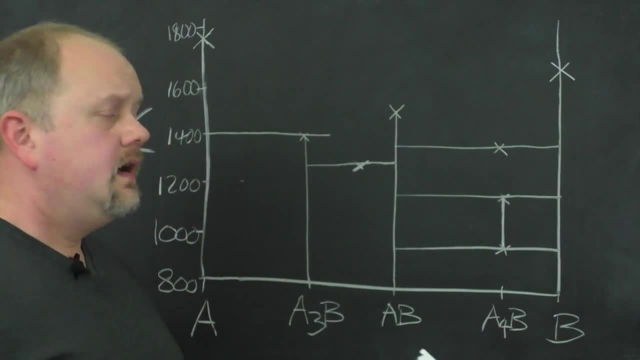 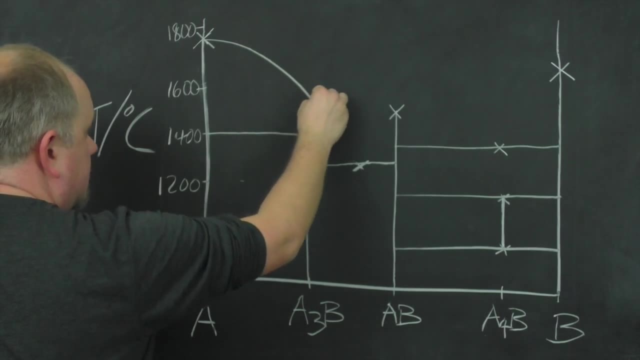 we know it's a eutectic so we can put another And then it's a simple case of joining the dots. So we know this needs to come down from A through the peritectic point here and onto the eutectic. We don't know from the information. 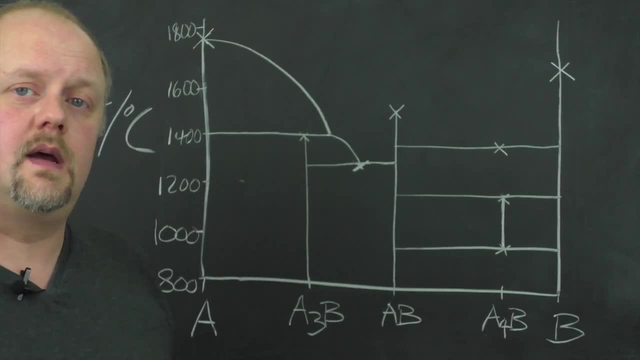 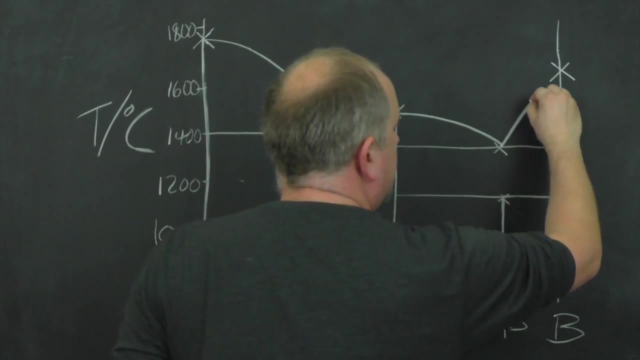 we're given exactly where this peritectic point should be. but it doesn't matter, We can make a reasonable guess and we won't be far off. And then it goes up to the congruently melting AB phase, To the next eutectic and up to B, And so we've got a reasonable shape for our eutectic. It might 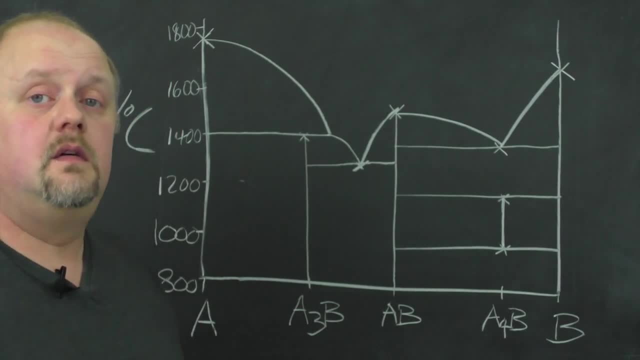 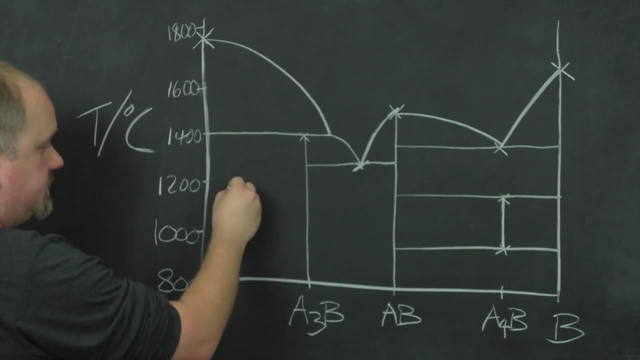 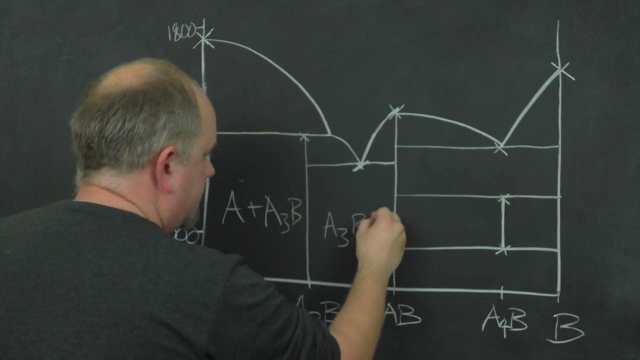 for our liquidus. sorry It might not be perfect, but it's a realistic shape. It's pretty reasonable guess And then we can just go through and label up some of these regions. So in here we have A plus A3B, A3B plus AB, AB plus AB. 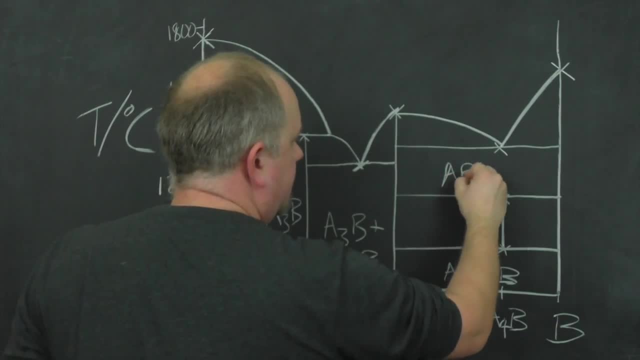 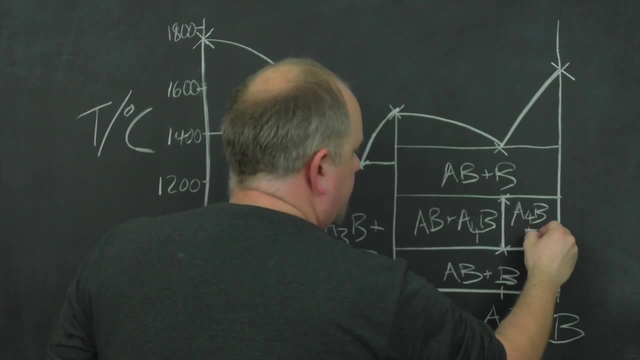 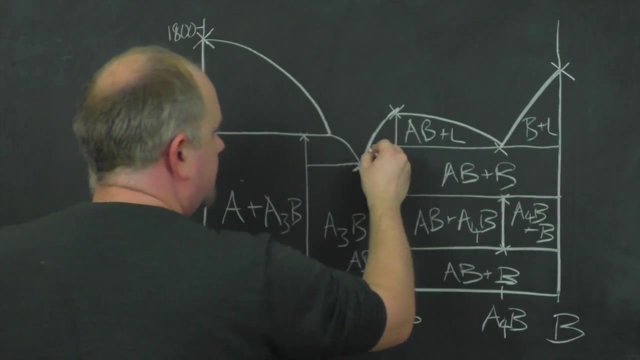 And in here we have AB plus B. That's the part that often catches people out. Down here we have AB plus A4B And in this lower region here A4B plus B, Then AB plus liquid, B plus liquid, A plus. 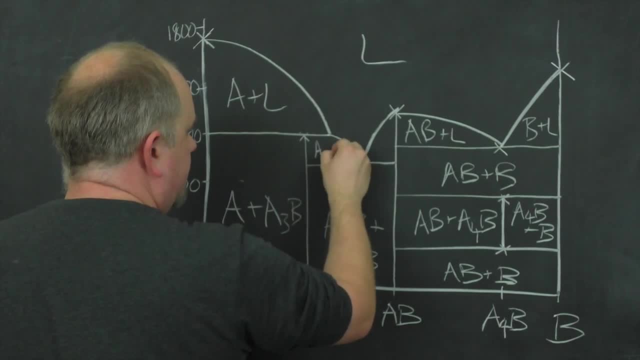 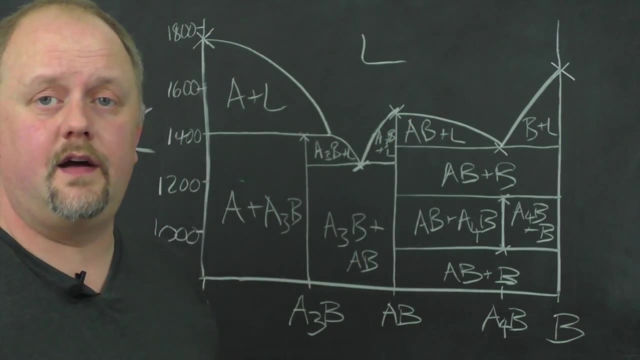 liquid: L Iquid at the top, AB, A, A plus liquid here and the same in here. So there you have a constructed and labeled phase diagram from a very brief description here.